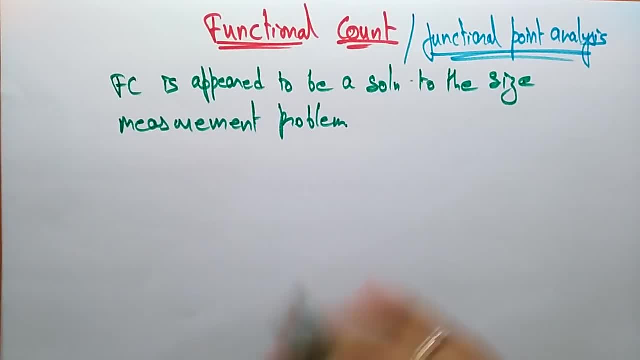 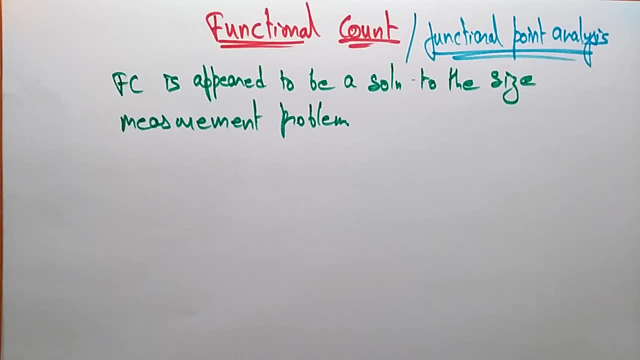 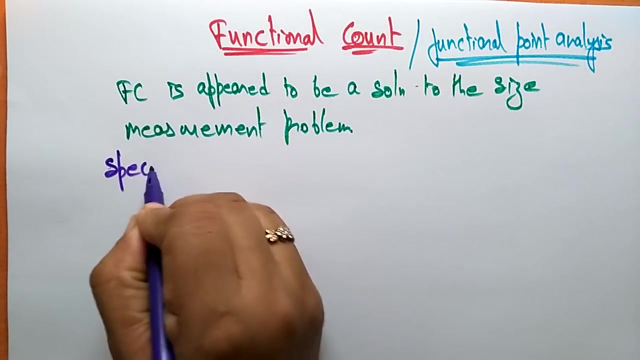 the program Means the input functions, output functions, internal functions, whatever If you want to deliver one product. So how many functions that is going to be undertaken, So that we have to be calculated? Now let us see the special features of this functional count. Special. 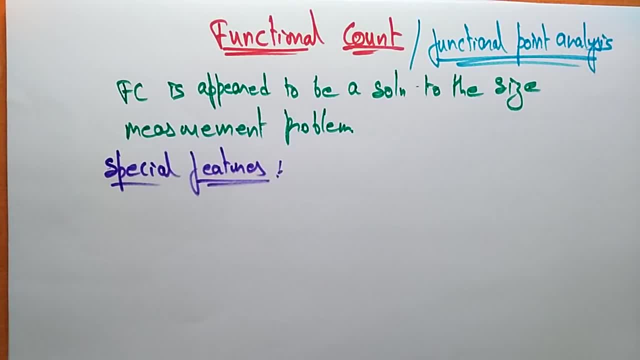 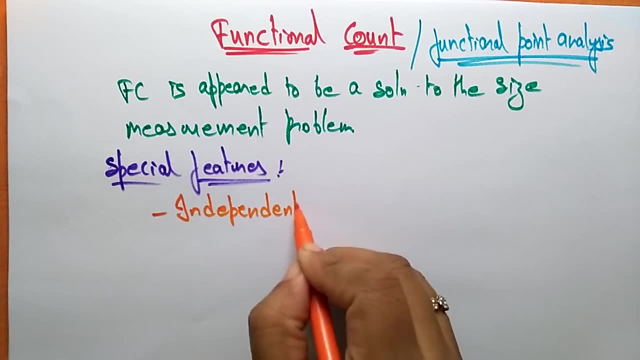 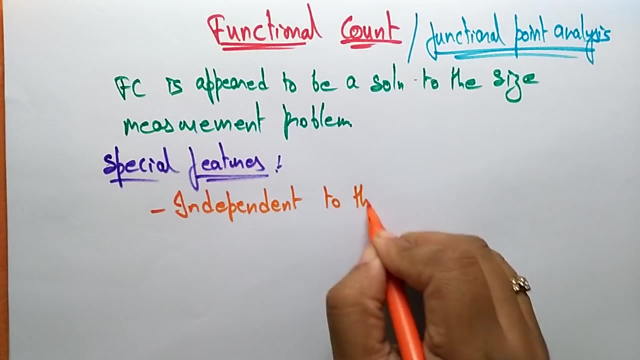 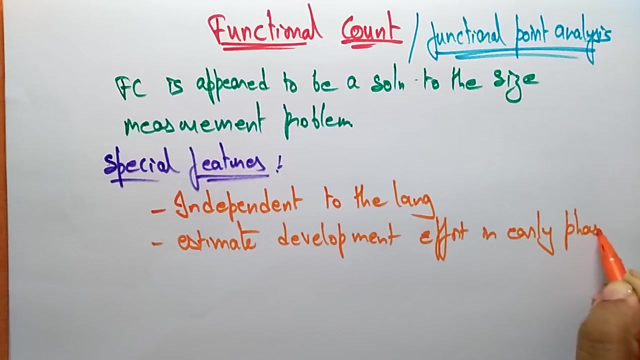 features, The special features Feature, or it is independent to the language, So it's not dependent in any type of language you can use. So for any type of language we can calculate the functional point analysis. So dependent, independent to the language, Estimate development effort in early phases. So in the early phases only we are going to be 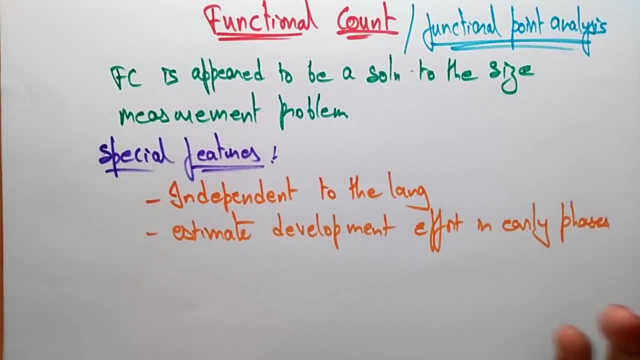 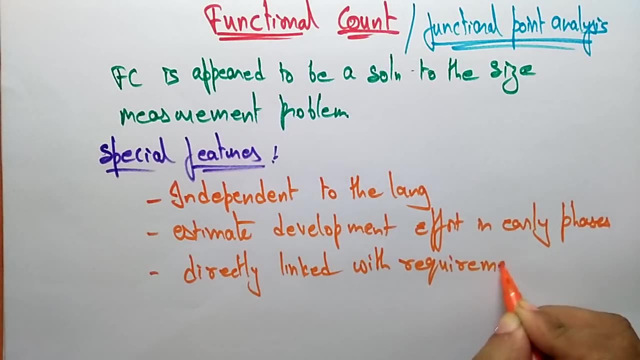 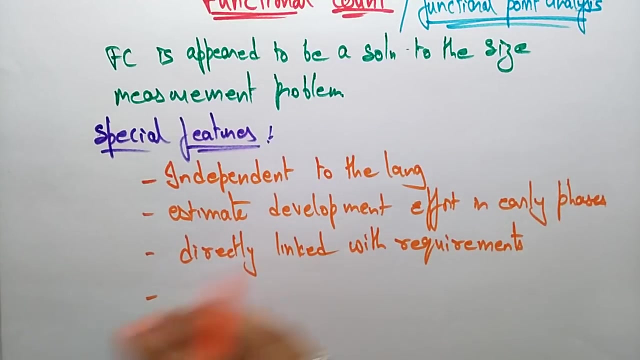 calculate The estimate development effort means how much the total effort that it takes to complete the process directly linked with the requirements. so this functional count and the functional point analysis is directly linked with the requirements so that we can easily calculate the functional point analysis if you know the all the related functions: information, the functional point. 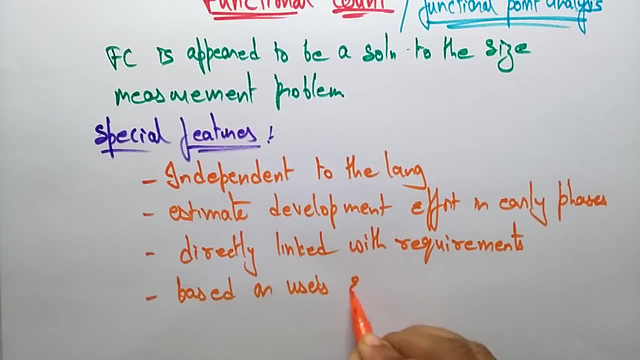 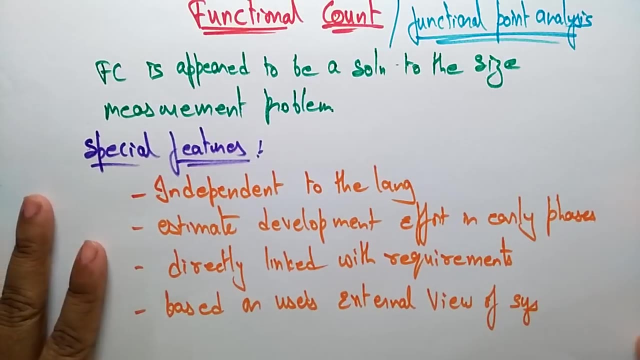 analysis based on users external view of system. so it is completely based on the user's external view of system. okay, now let us see what exactly this functional, the principle of this functional point analysis. so let's see explain about the features. now let us see the principle of 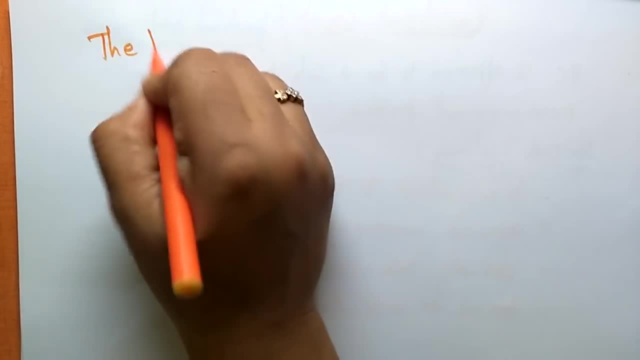 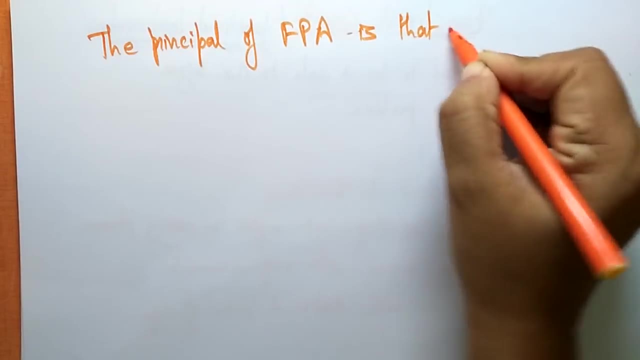 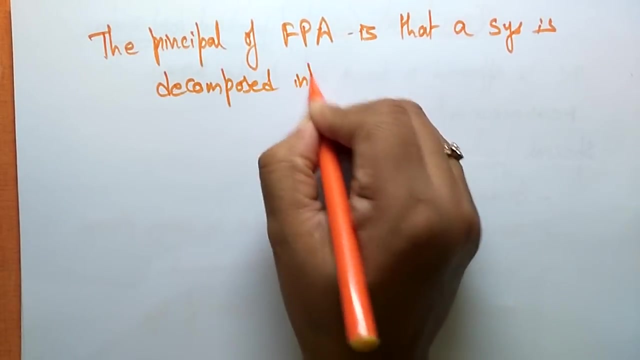 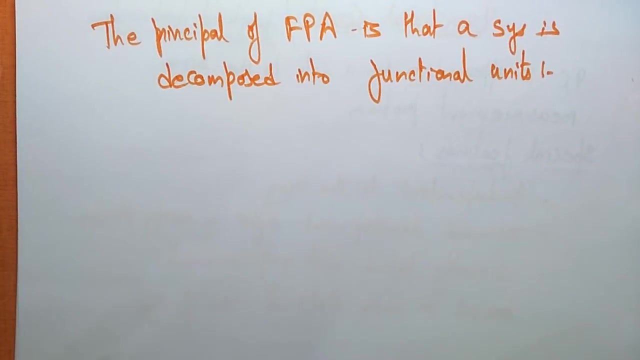 functional point analysis. the principle of the functional point analysis is that a system is decomposed into, decomposed into functional units. so if you take any system, if you take any system, that system will be decomposed into functional units. the main, the the principle of this functional point analysis is to decompose the system into functional units so totally. 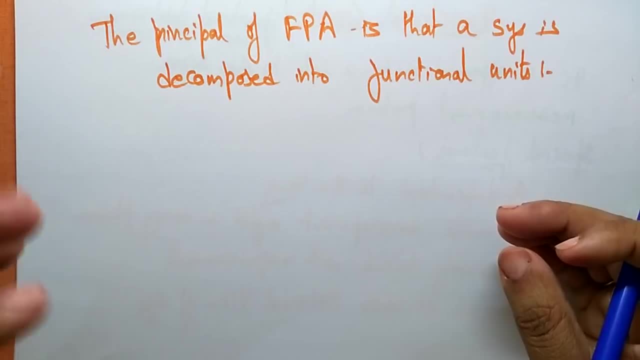 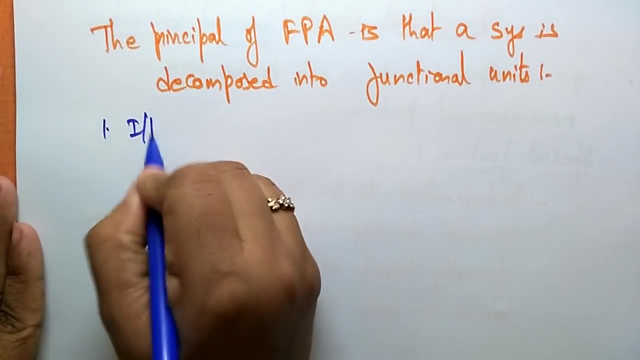 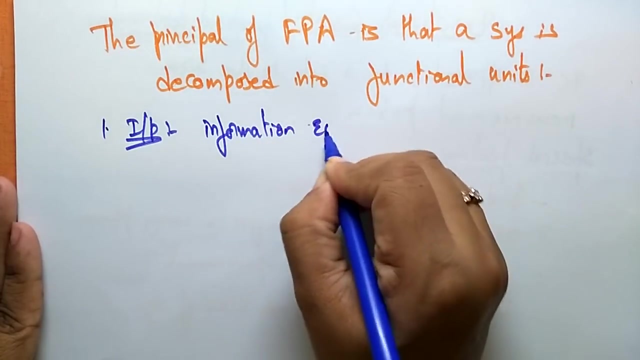 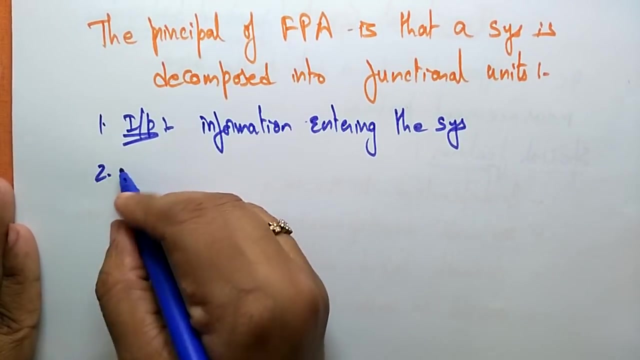 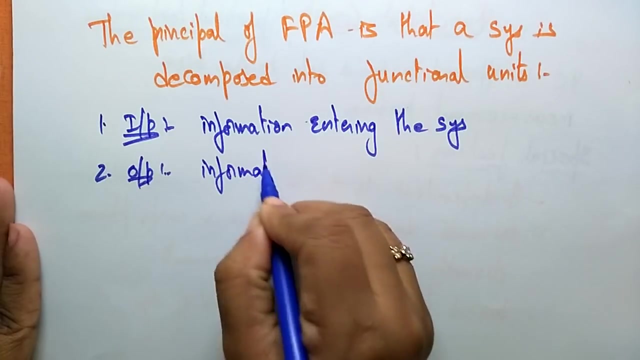 are five functional units that are present in the that will be decomposed. the system is decomposed into five functional unit. the first thing is input. input here information, information entering the system. we call it as an input- here we are entering the information into the system. and output: output means information leaving the system, information is leaving out from the system. 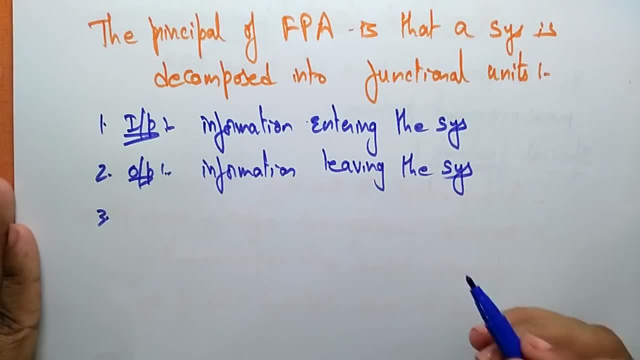 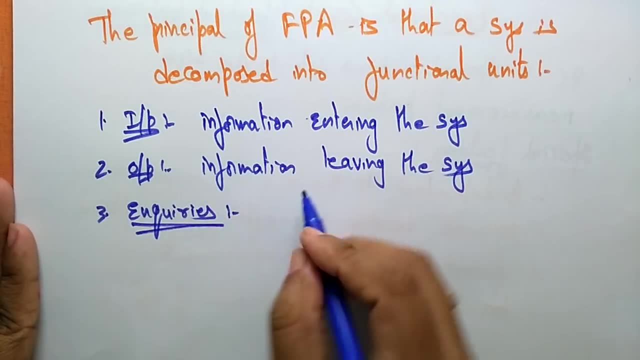 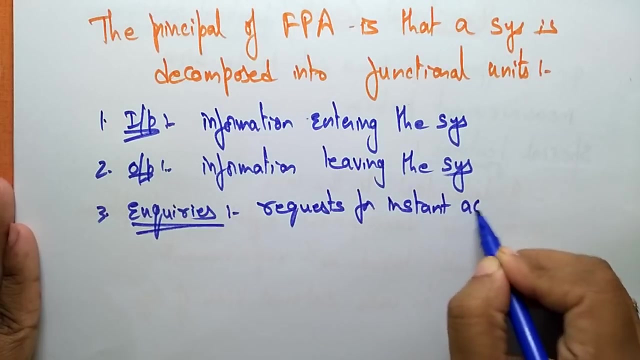 leaving the system. and the third functional unit is a enquiries. enquiries is related to both input and output here the request for instant access information. so whether it is an input or an output, we have to just request an access for an instant access information inside the system or outside the system and internal logic files. 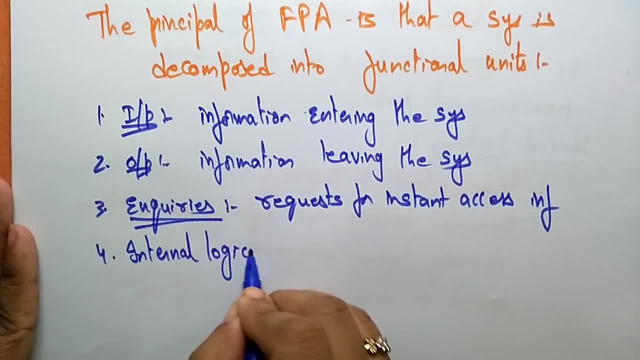 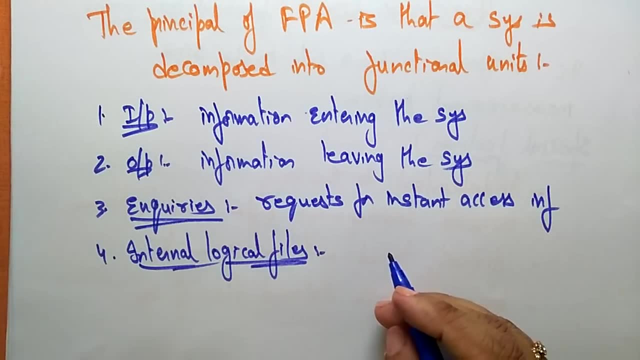 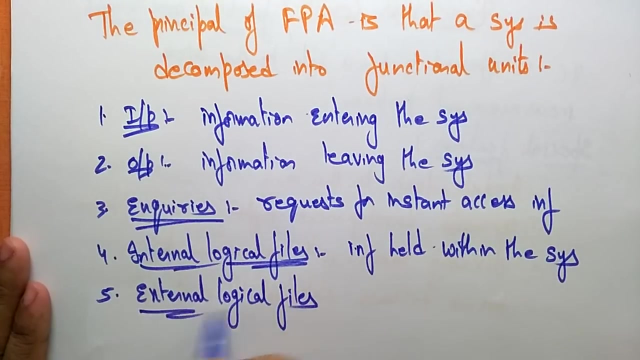 internal logical files. internal logical files means information held within the system. you call it as an internal logical file- the logical files that are present inside the system. then you call it as internal logical files- Information held within the system- and external logical files- External logical files. 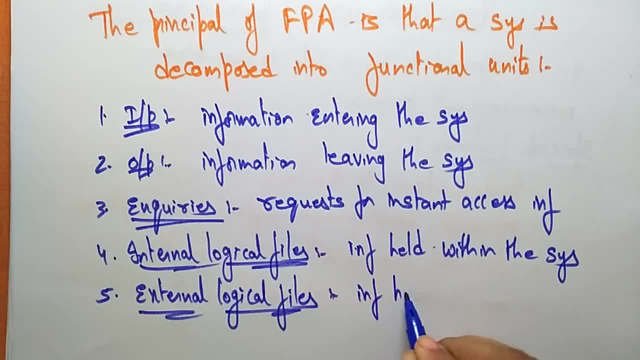 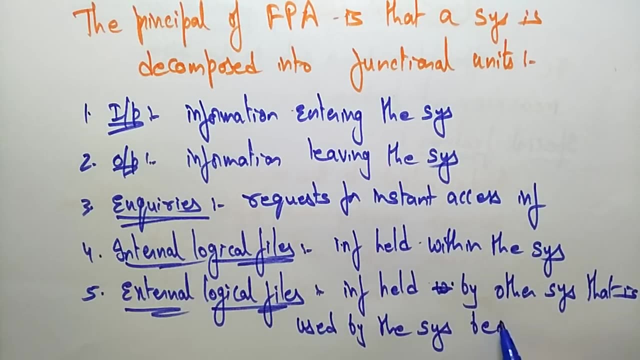 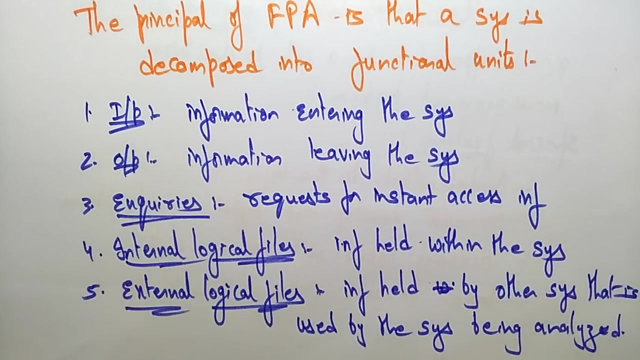 So here, information held by other system that is used by the system being analyzed, System being analyzed. So these are the 5 functional unit. A system is decomposed into 5 functional unit, So this is the main principle of the functional point analysis. 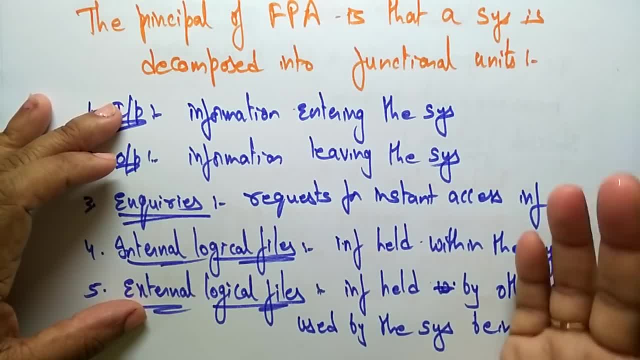 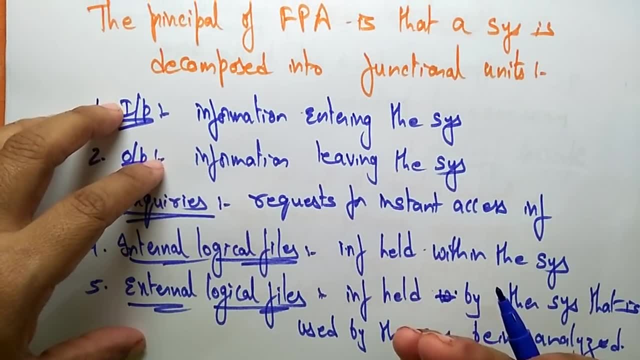 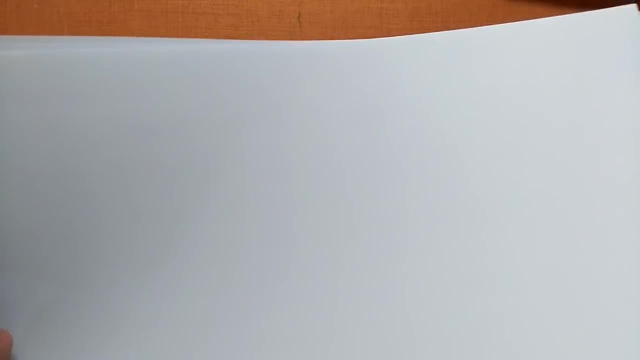 If you want to calculate the functional point analysis, you have to divide the system into five functional units: input, output, inquiries, internal logic, external logic. so with the help of these functional units you can calculate the functional point analysis of your system. okay, so these five functional units are categorized. 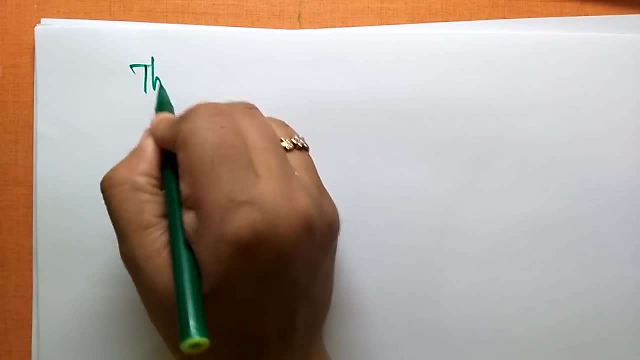 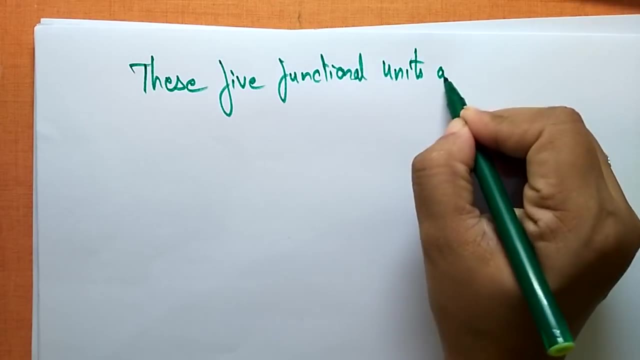 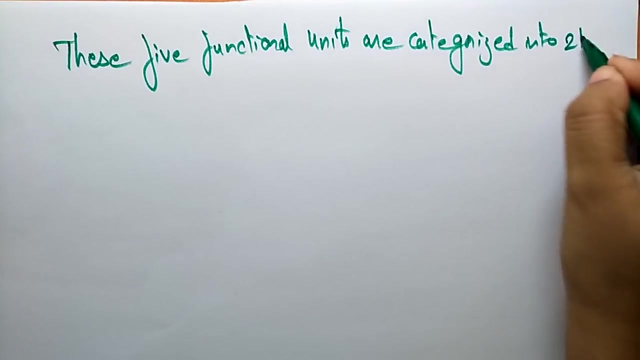 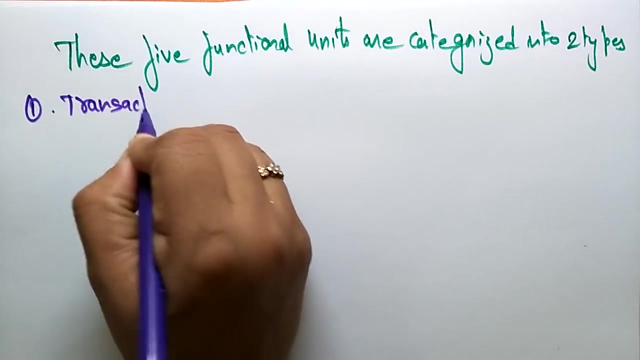 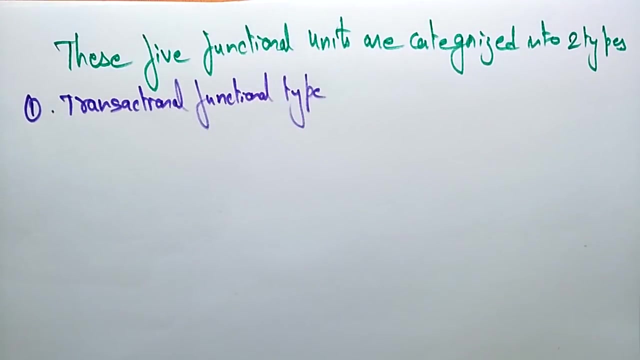 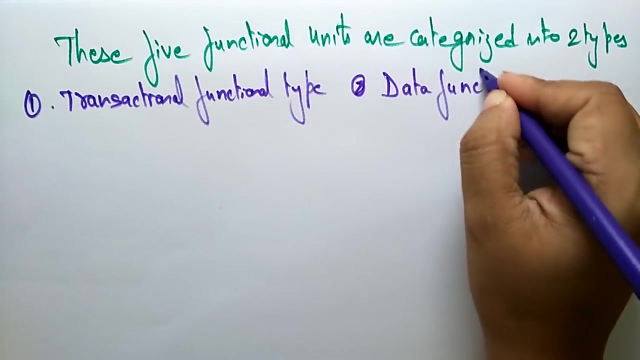 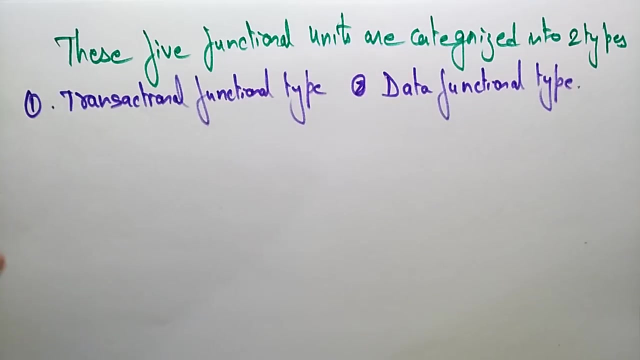 into two types again, these, these five functional unit, or categorized into, categorized into two types. so one is transactional functional unit, functional type, transactional functional type, and the second one is data functional type, data functional time. so this five functional units, that is, input, output, enquiries, internal logic. 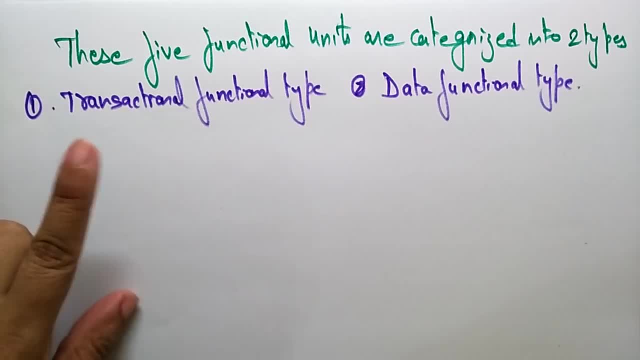 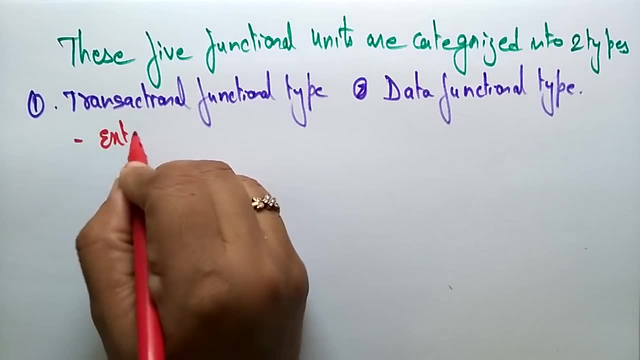 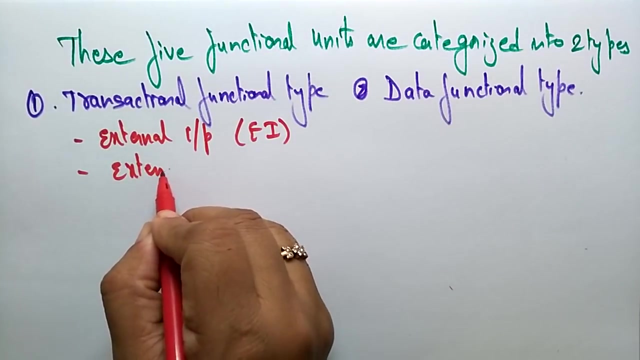 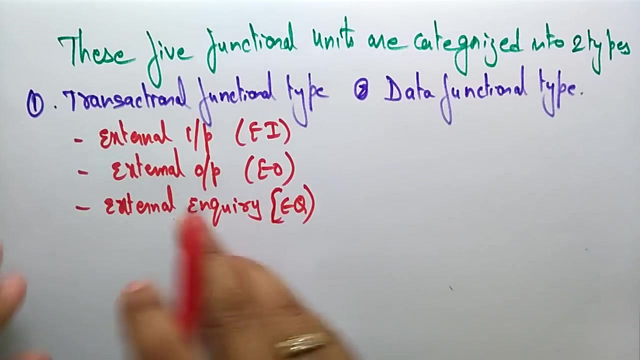 external interface files are divided into two categories: transactional functional type and the data functional type. transactional functional types are nothing but the external input, equal it as e I, external output, Evo and external inquiries, external inquiry, that is EQ. so these three comes under the transactional functional type. we are 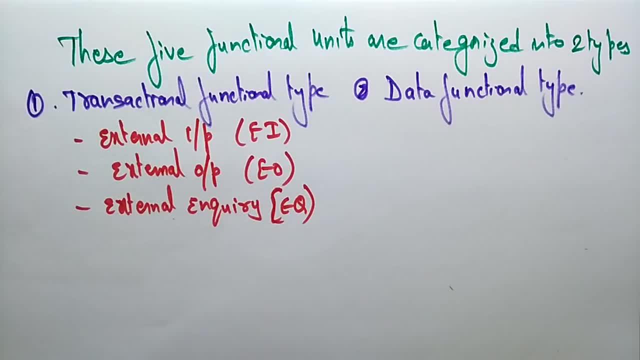 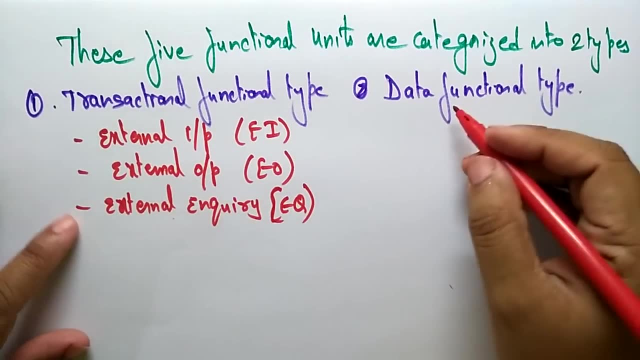 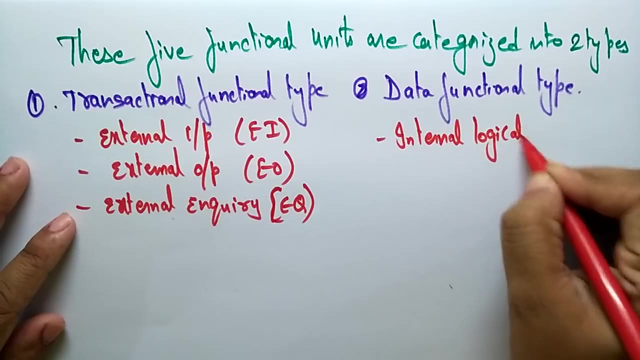 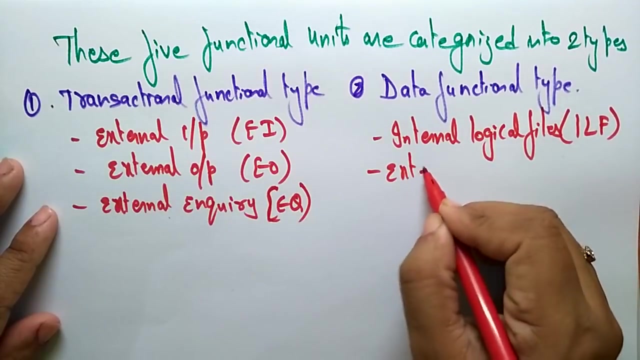 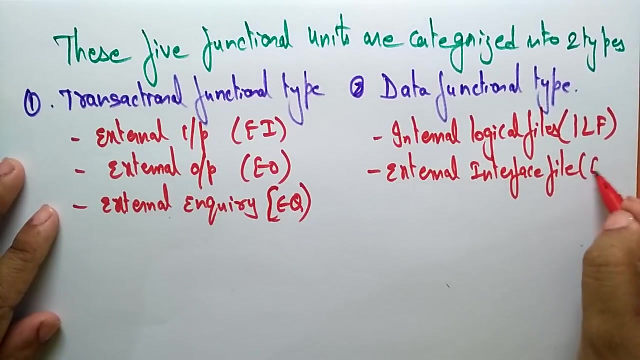 transaction with data. we are transaction the functions, so we have to calculate that function. point answers also external input, external output, external inquiries. then what about the data functional types? data functional types or comes under the internal logical files- we call it as I, L, F and external interface files. so these two comes under the data functional type, here the data. 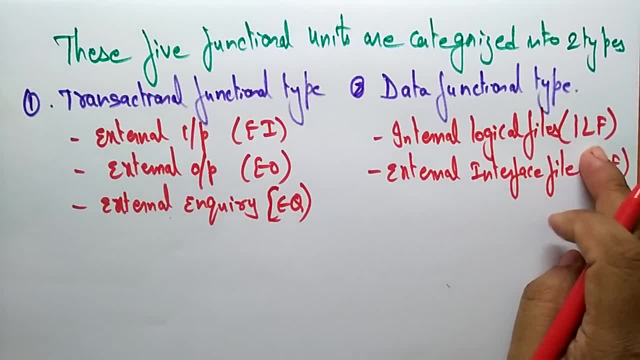 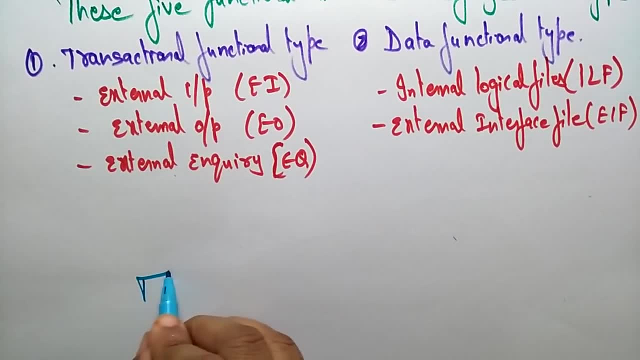 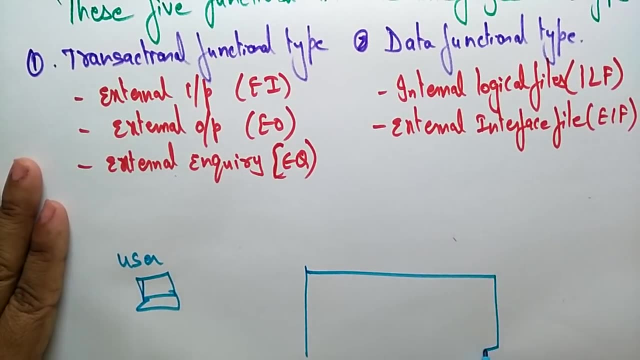 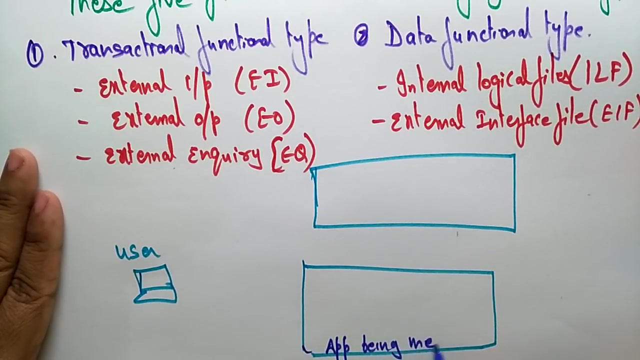 information will be passed: internal logical files- I LF- and external interface files. so now let me show you the simple diagram. so here a user was there. let us take this is a user. okay, so here we are having. this is application being measured. here let us take application being. 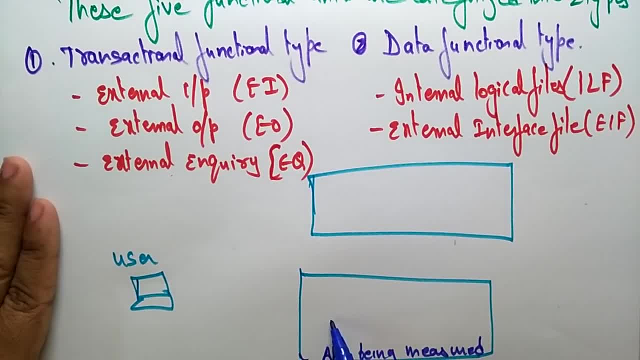 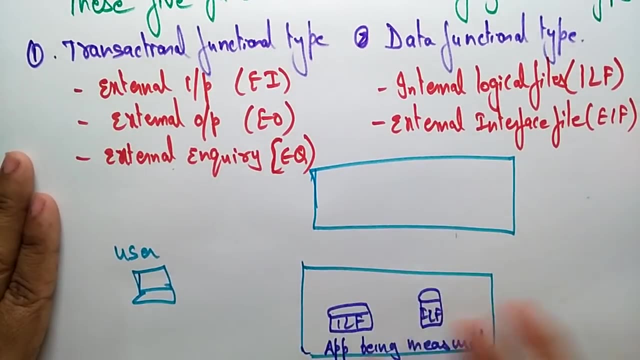 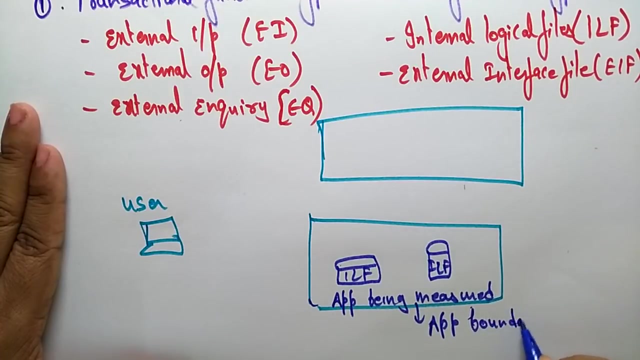 measured in this area and it consisting of some internal logical files, ILF, ILF, so ILF- internal logical files are present in this application boundary. we call it as an application application boundary. so in this application boundary you are having the internal logical files. all logical files are present in this. 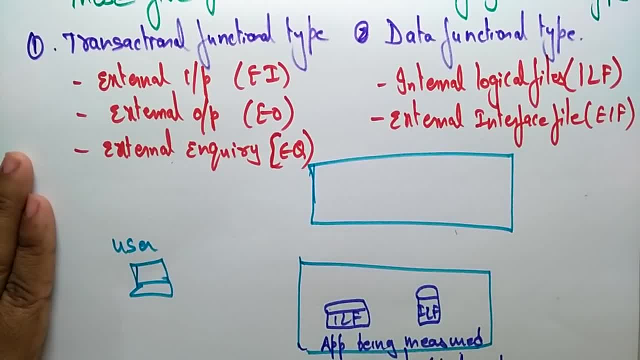 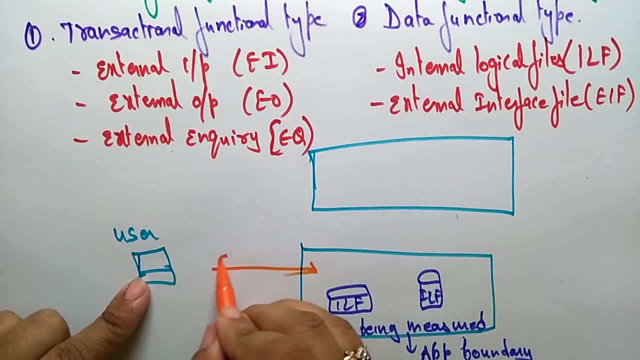 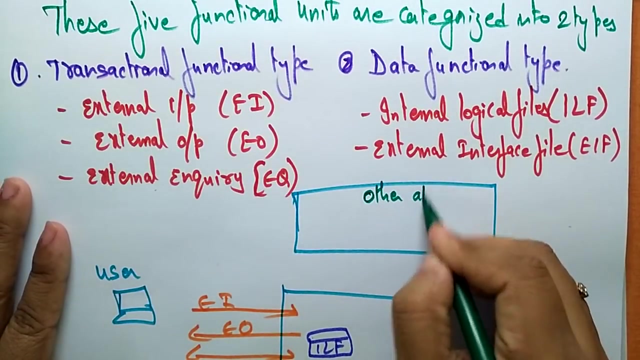 disks and Here is a communication, so the user is communicated to this application boundary, like it gives an external input, external output, and this is a bi-directional of external inquiries, input and output. okay, and here you are having the other applications, some other applications. so like hard disk URL, like Arabic domain, like a standard risk, and 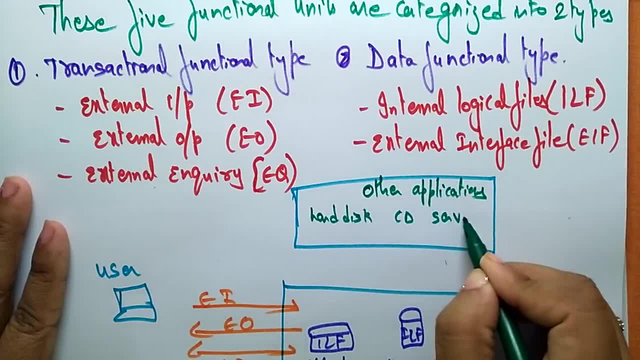 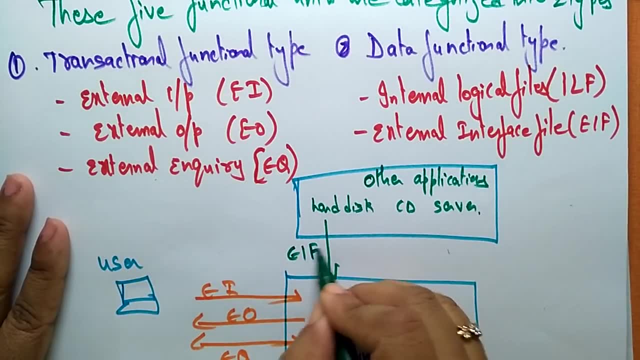 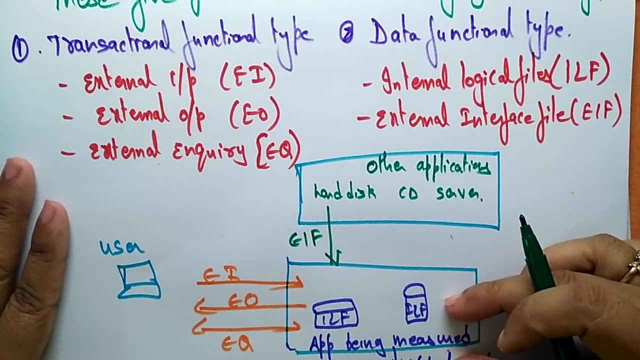 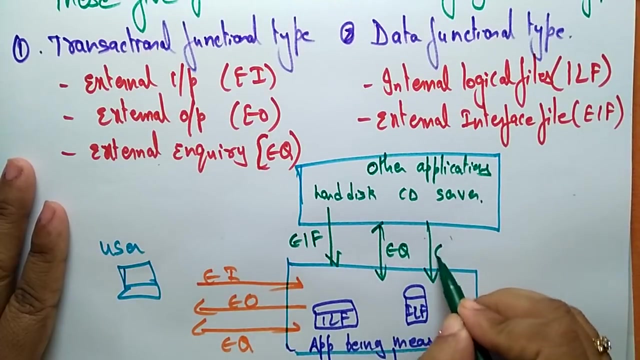 cds, servers, apps, different other applications will be there, so this will be communicated with this external interface file. so this is an external other applications, these are other applications are interfacing with the application boundaries, that is, external interface file, external queries, external input, external output. so for the other applications also, these will be. 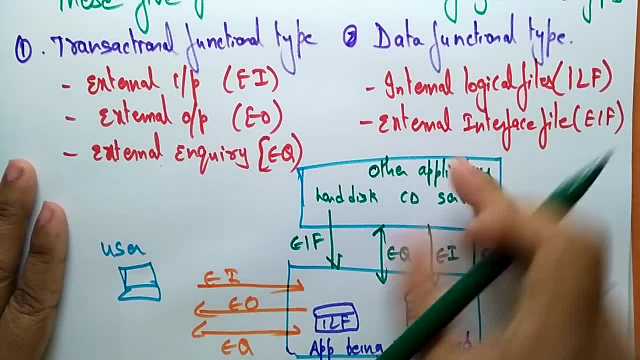 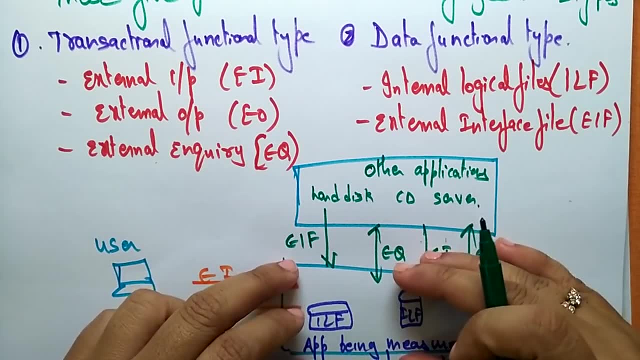 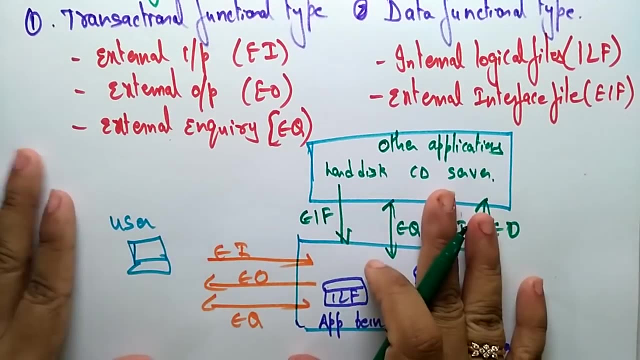 giving input, taking the input and giving the output. okay, so this application boundary is interfacing with the user and the other applications. so this is a main server. so this is interacting with the users and with the other applications. so, and these are all the some functional units that are present in the application boundaries, so this is a main. 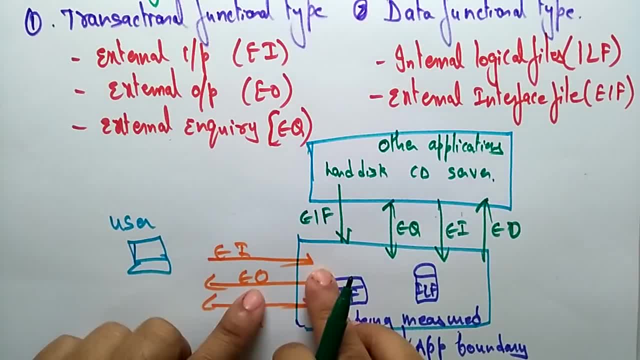 to perform the actions: external input, external output, external queries, external interface file in internal logical files. so we have to calculate all these by, with the help of these all functional units, we have to calculate the functional point analysis, that just adjustable functional point analysis. okay, so that I will explain with an example in the next video. thank you.